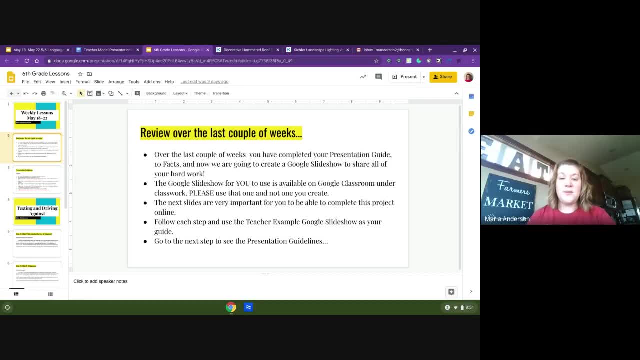 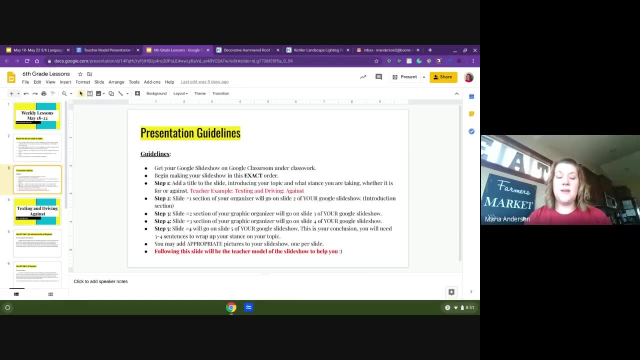 Please do not make one create your own. Use the resources that we are providing for you. It also is really important for you, this next part of the lesson, to follow the guide in exact order. So meaning if I were you, I would do step one and then on yours, and then step two, just to keep it in order. 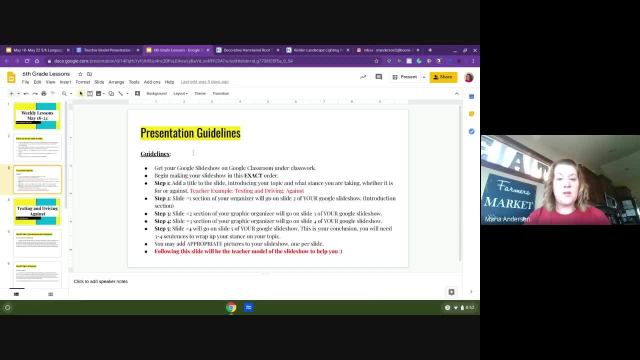 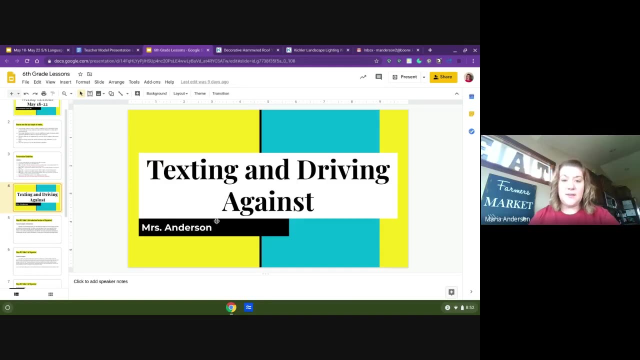 because there's quite a few steps with this. So, step one: you're going to add a title introducing your topic, what stance that you're taking, whether it's for or against. So the teacher example was driving or texting and driving against. So in the next slide you can see there is texting and 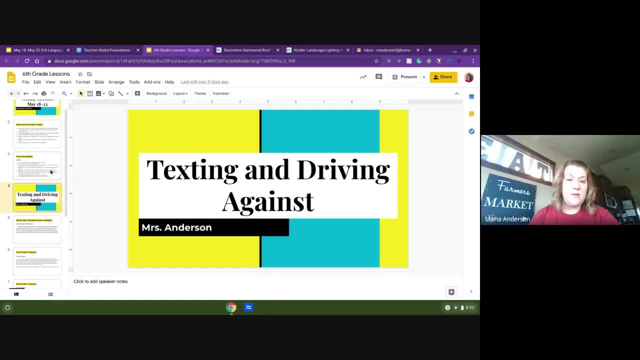 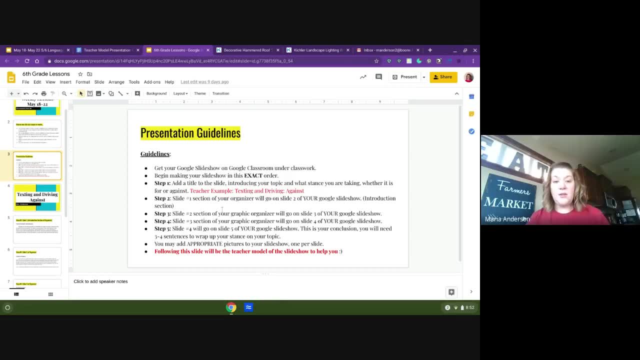 driving against, and then my name. So you need to do the same thing. Your slideshow: it will look exactly like this. So that's your slide one. Now slide two is section one of your organizer. Here's where it gets tricky. So meaning when you go to your presentation guide. 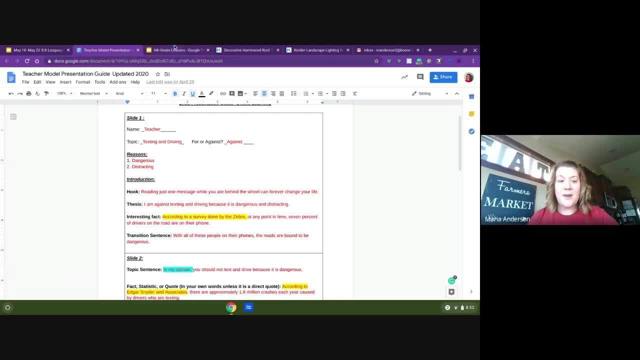 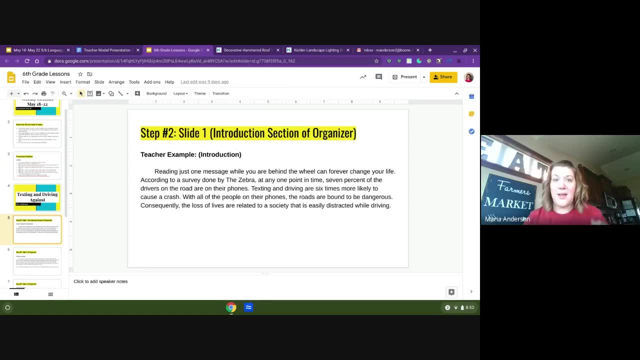 here is slide one. that's the top part. That information is going on slide two, or step two, which is slide two of your presentation, And you're going to want to put it in paragraph order. So that's what I did with this, So reading just one message while you are behind. 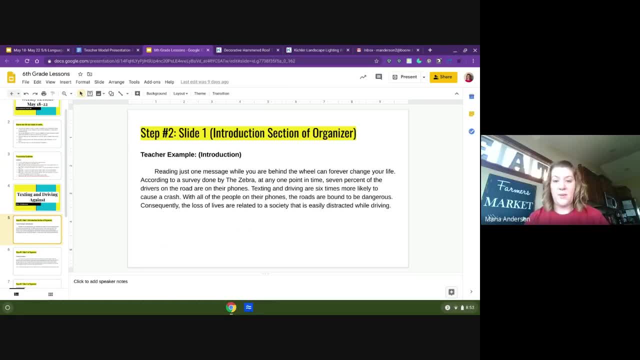 the wheel can forever change your life. According to a survey done by the Zebra, at any one point in time, 7% of the drivers on the road are on their phones. Texting and driving are six times more likely to cause a crash. With all the people on their phones, the roads are bound to be. 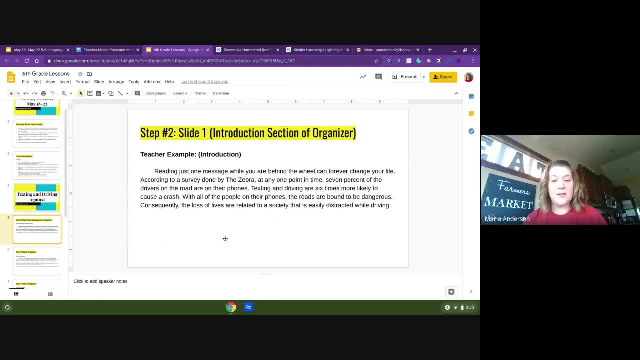 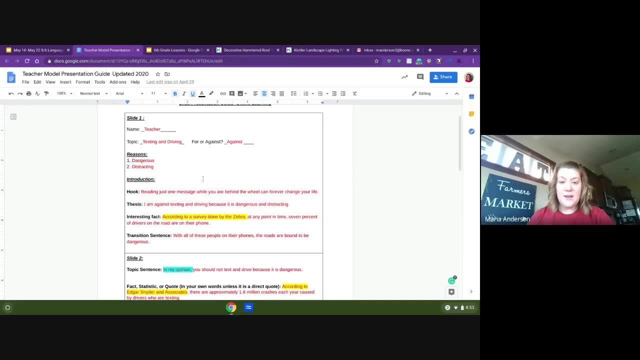 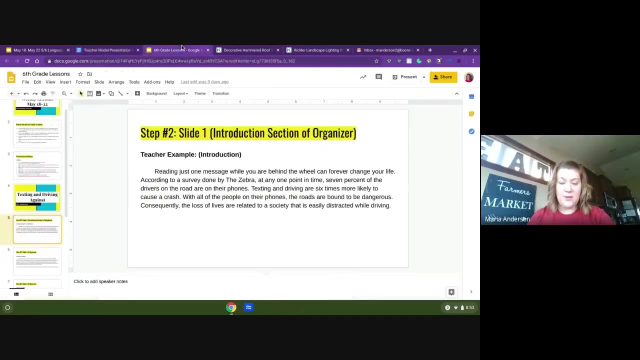 dangerous. Consequently, the loss of lives are related to a society that is easily distracted while driving. So that's what I did with this: So reading just one message while you are behind. So, if you remember, that is coming from all of the information on slide one of the teacher model. 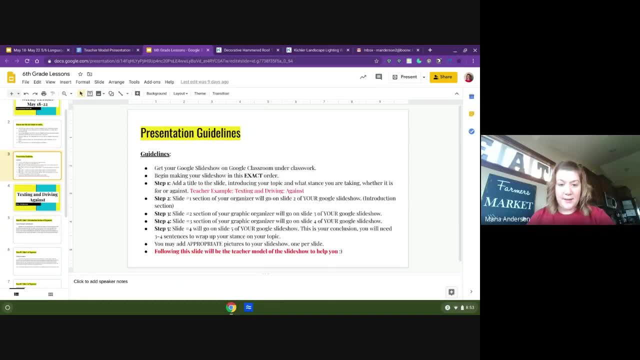 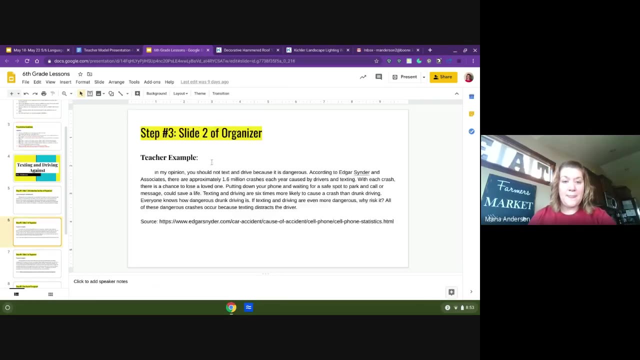 So go back to that if you need it. So back to the guidelines. So step three is going to be slide number two, section of your graphic organizer. So this here's my example. So this is step three, slide two. these all match your directions. So if you get confused, take a look at what slide. 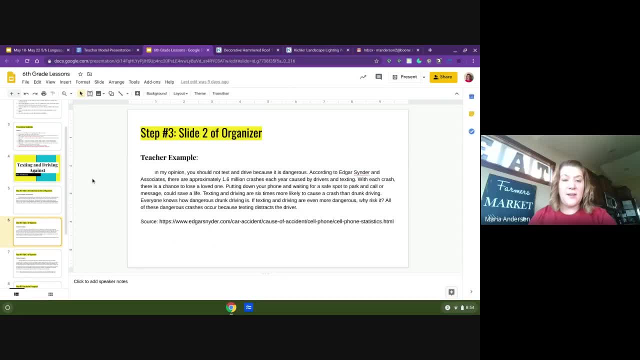 you're on and go back to that presentation guidelines. So here is slide two of my organizer showing up on step three. Okay, So this talks about this. Here's my example. In my opinion, you should not text and drive because it's dangerous. I give all the information from: 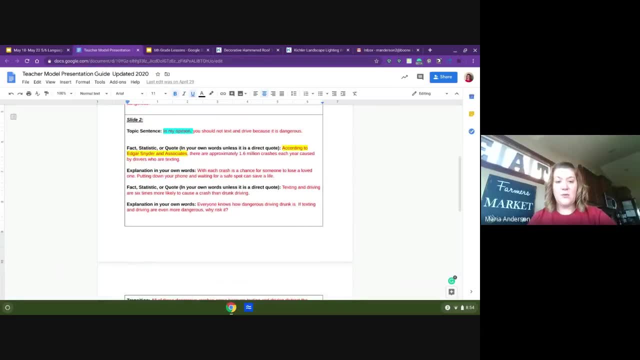 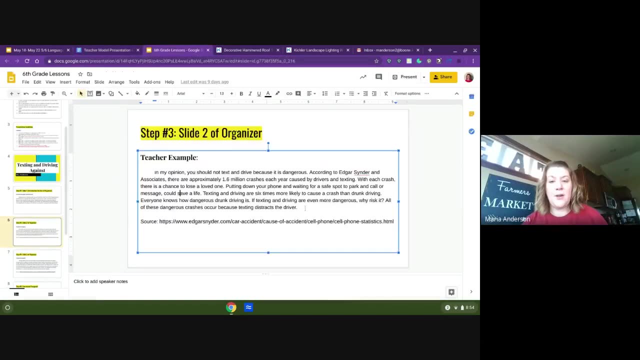 slide two, which is right there. Take all of that information and put it into a paragraph, put it on your slide and then copy and paste your source. Just do it right on the bottom list: a source. Okay, Then the same thing with the next one Step. number four is slide three. 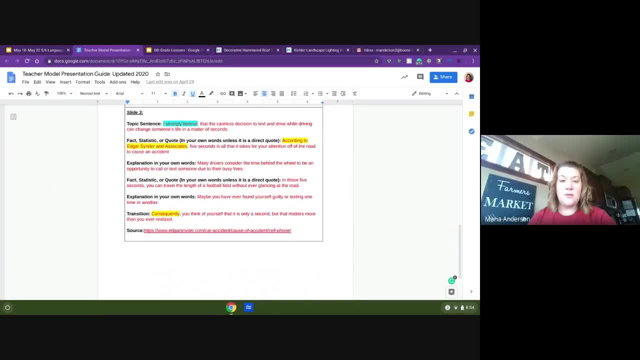 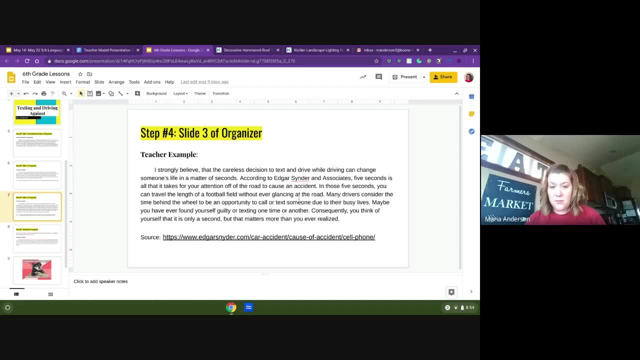 of your organizer. Okay, So go down to slide. three of your organizer take all of that information, put it into a paragraph, put it on your slide and then copy all of that information that you have there, turn it into a paragraph, So you might have to add: 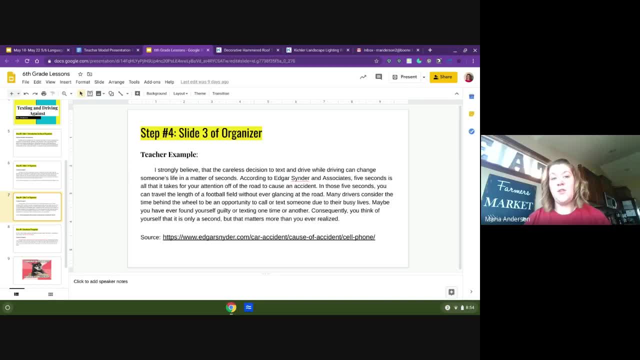 a sentence depending on what types of information you put on your presentation guide. So keep that in mind. Remember: a paragraph is three to four sentences, So I want to make sure that you understand that these need to look like a paragraph, not that you are just putting facts down. 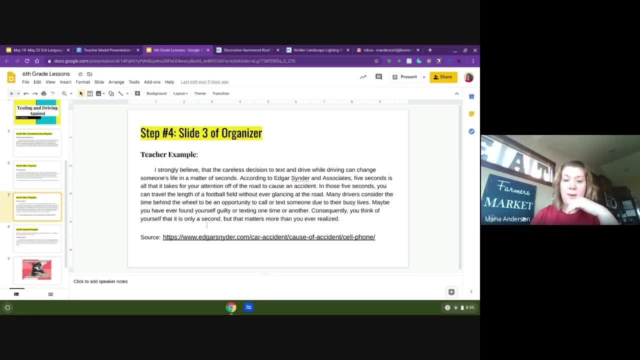 because we've already done that. Okay, So here's my presentation, So I'm going to go ahead, and here's my paragraph, And then again there's the source. So just copy and paste it, put it on your slide, So that way we know that you have a source for it. Well, here is step number five. This is: 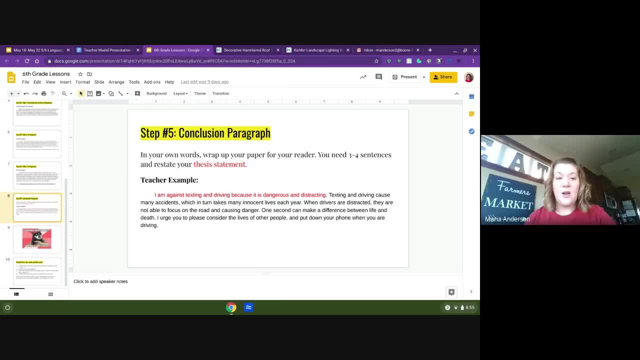 the conclusion paragraph. You did not do this on your graphic organizer, So this is something you're going to have to do on your own. So, in your own words, you need to wrap up your paper for your reader. Nothing different than we've ever done. You need three to four sentences and 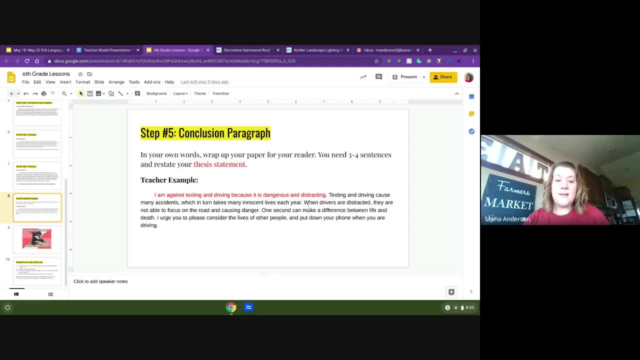 restate your thesis statement. Okay, That's important when you are wrapping up, especially when it comes to a persuasive paper. Okay, So there's my thesis statement in red. I am against texting and driving because it is dangerous and distracting If you do not remember where your 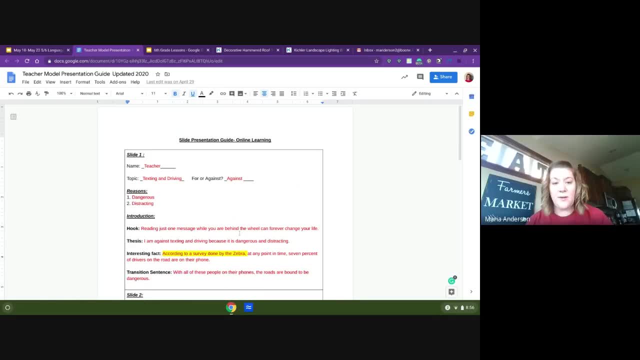 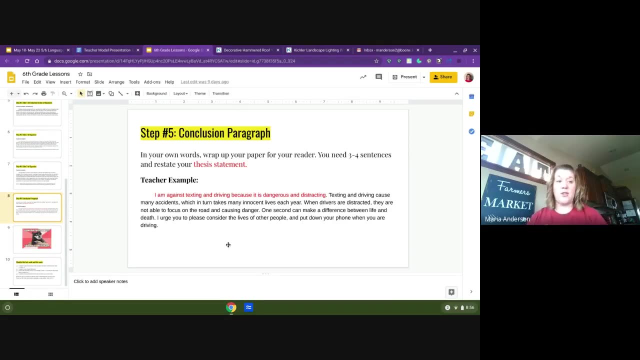 thesis statement is. it is right up on the top of slide one, right after your hook, So go back to there if you can't remember by chance. or it should be in your introduction paragraph in the beginning of this slideshow. Okay, So you need to come up with a paragraph. 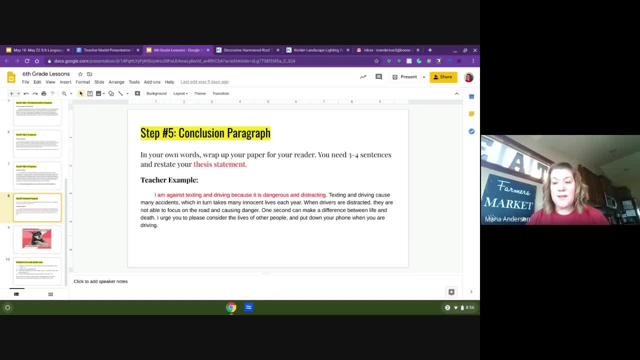 wrapping up your paper, So mine ends with texting. and driving cause many accidents, which in turn takes many innocent lives each year. When drivers are distracted, they are not able to focus on the road and causing danger. One second can make a difference between life and death. 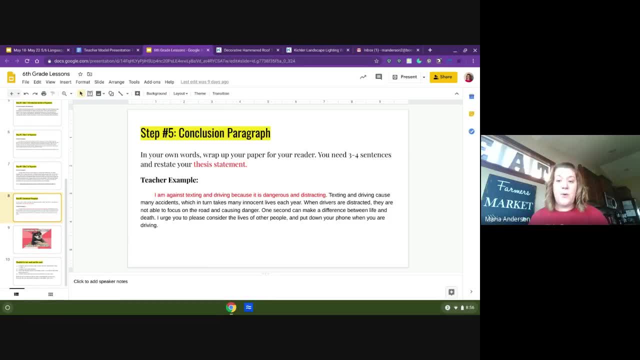 I urge you to please consider the lives of other people and put down your phone when you are driving. So I am persuading you to consider the lives of other people and put down your phone when you are driving. So I am persuading you to consider the lives of other people and put down your phone when you are driving. 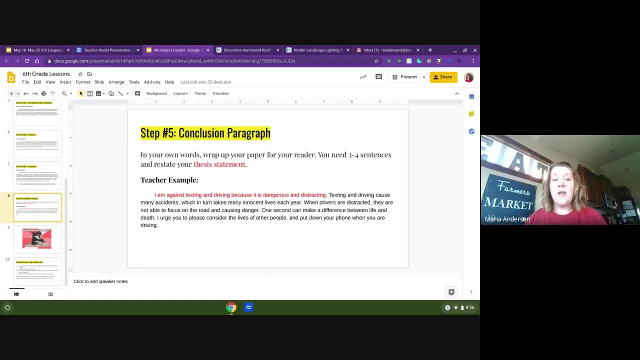 So I am persuading you to consider the lives of other people and put down your phone when you are driving. Remember you are persuading somebody to either agree with you or disagree. So make sure that your conclusion, you end it boldly, Okay. 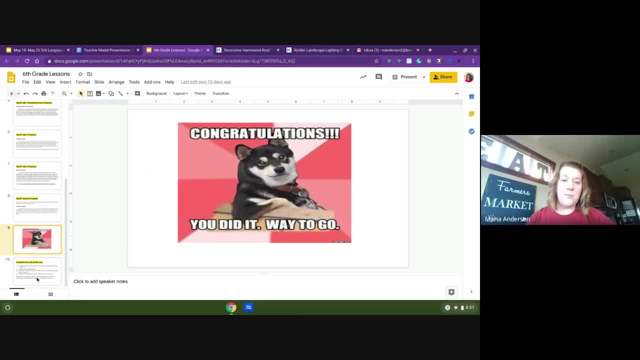 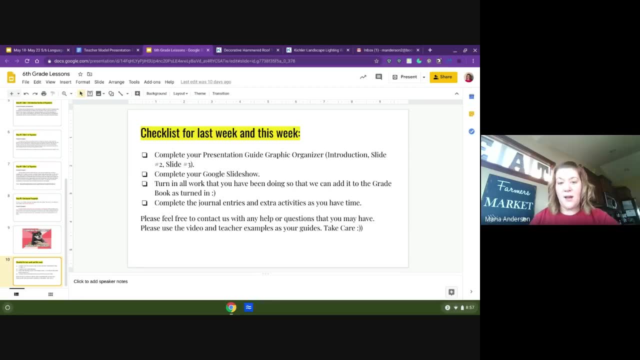 And congratulations. We did it. We survived the persuasive unit right. So here's our checklist, just to kind of remind you things that we are needing to add into Infinite Campus, The first one being your presentation guide graphic organizer. Once you're done with your slideshow, you should be able to turn that in. You won't need it anymore. 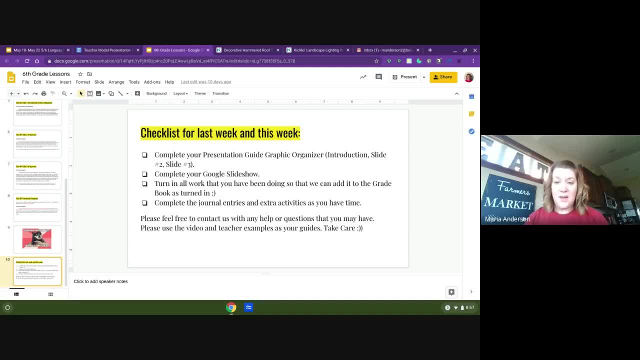 Make sure, once you're done with your slideshow, you turn that in And then also, if you forgot, to turn in your 10 facts. So that way, for the continuous online learning in the persuasive unit, you should have three assignments in Infinite Campus. At least that's the goal. So. 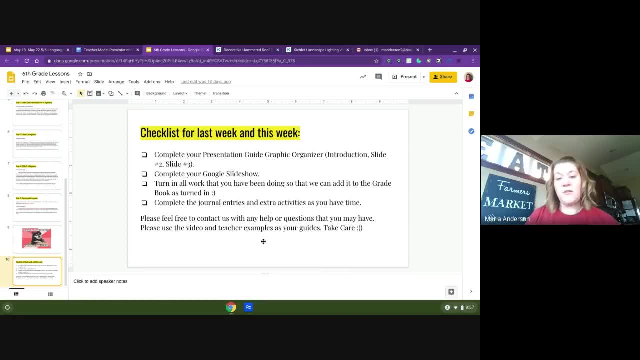 if you have any questions, please make sure that you reach out Video chatting with us on Tuesday and Thursday. Ms Kelly and I and Mrs Morris are all three available on Tuesday and Thursday from 9 to 11. But we are talking every day, So if you guys need something, it's really easy for us to. 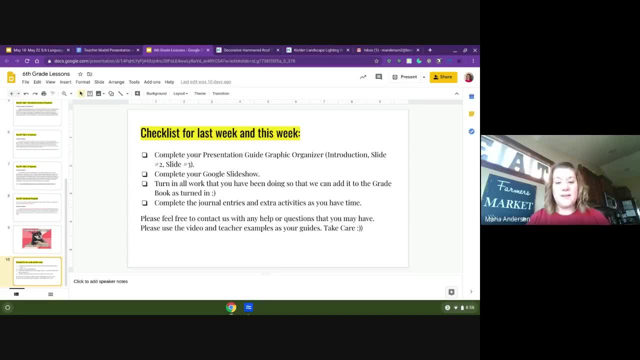 jump on and help you out, Okay, So yeah, You guys take care of yourselves and I will see you next week.